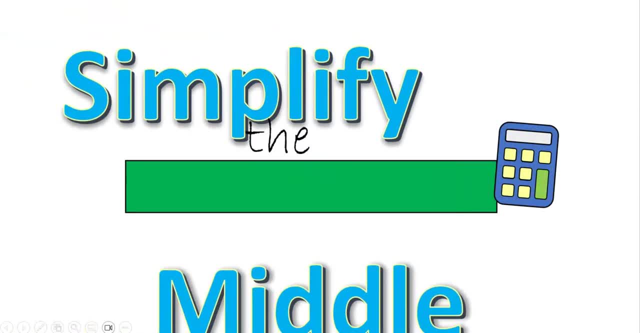 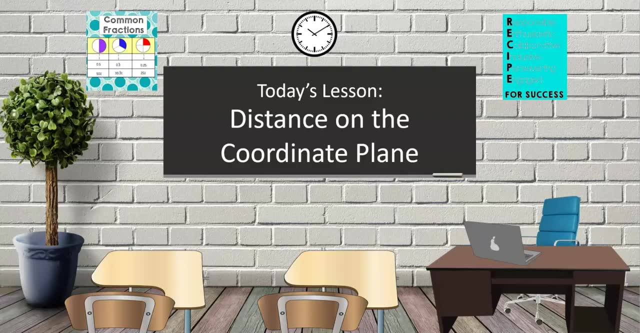 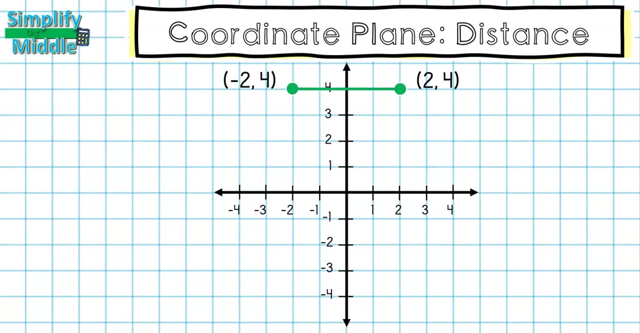 Hi and welcome to today's lesson: distance on the coordinate plane. Here we have a couple of points. Today we will learn how to find the distance between points like these, but first we need to identify if a line is horizontal or vertical. This line is an example of a horizontal line. 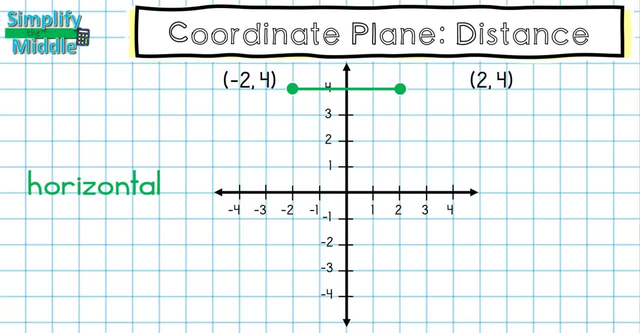 Let's look at Y. If we were to stack our two points on top of each other and we look at the x-coordinates and the y-coordinates, we notice something: Our Y-coordinates are both 4.. So whenever we have the same Y coordinate, we know we are talking about a horizontal. 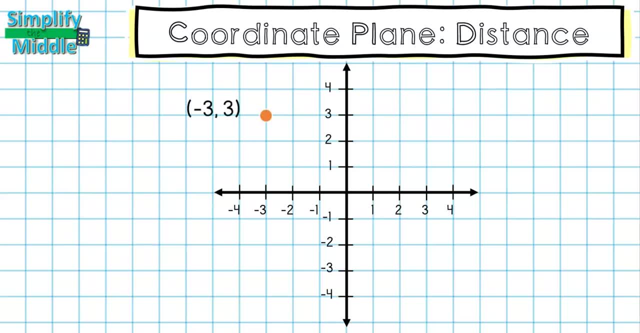 line. Let's look at a couple of other points. Here we have- and This is an example of a horizontal line, And here is a example of a horizontal line- On the other hand, we have distractor coordinates, So we can see that both horizontal lines have horizontal coordinates on top of each other. 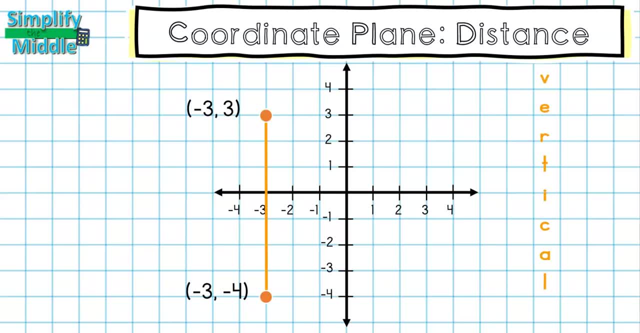 vertical line because it is straight up and down. If we take a closer look at our ordered pairs, we notice something about our coordinates again, In this one we can see our x-coordinates are both negative 3. So anytime that two ordered pairs have 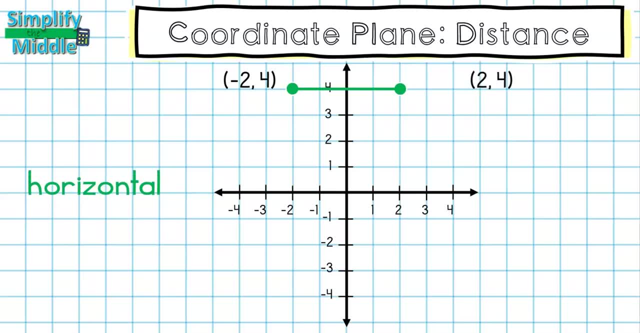 Let's look at y. If we were to stack our two points on top of each other and we look at the exchange coordinates and the y-coordinates, we notice something: Our y-coordinates are both 4.. So whenever we have the same y-coordinate, we know we're talking about a horizontal. 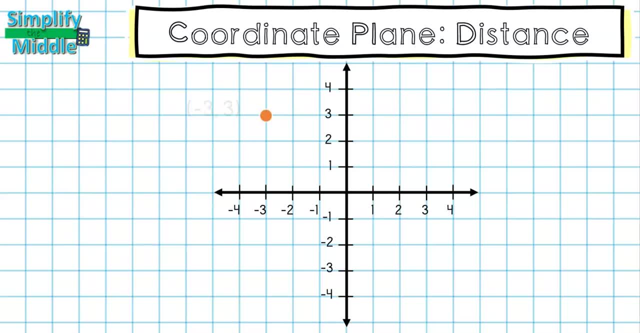 line. Let's look at a couple of other points. Here we have and- and This is an example of a분 vertical line because it is straight up and down. If we take a closer look at our ordered pairs, we notice something about our coordinates. again, In this one we can: 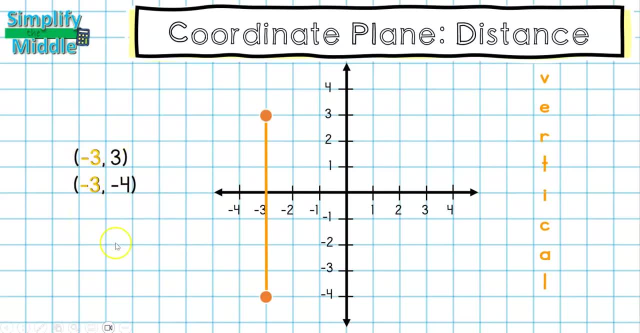 see, our x-coordinates are both negative 3.. So anytime that two ordered pairs have the same x-coordinate, they make a vertical line. Now that we understand the difference between them, let's practice trying to find the distance between them. So here I have two points: 1, 4, and 4, 4.. I automatically know that they are. 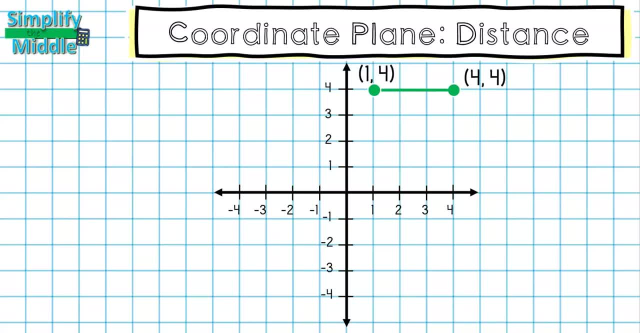 horizontal because I see them graphed. But what about if I don't see them graphed? So, because these ones are graphed, I do notice that it is going from left to right and I also can see from my ordered pairs. if I didn't have a picture of it, I 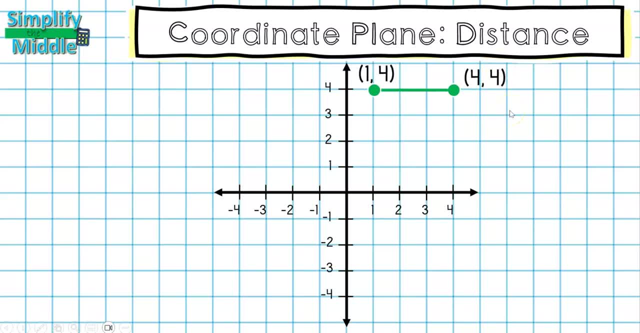 can see from my ordered pairs that the y-values, the y-coordinates, are the same. This means horizontal. Now to find the distance in a picture, I can just count it The distance between them. So this is 3.. So let's try another way to find the. 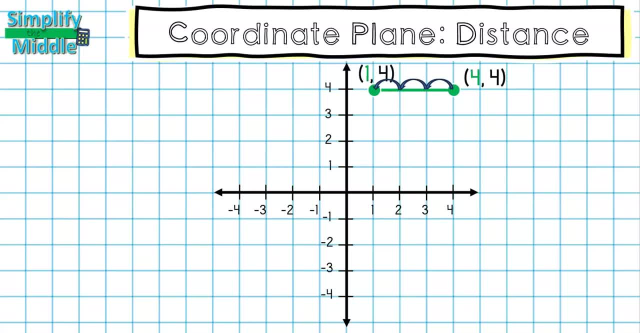 distance when I don't have the picture. So if I was to just have the ordered pairs To find distance, we're going to look at the coordinates that are not shared, In this case the x-coordinates. We will take the larger minus the smaller. 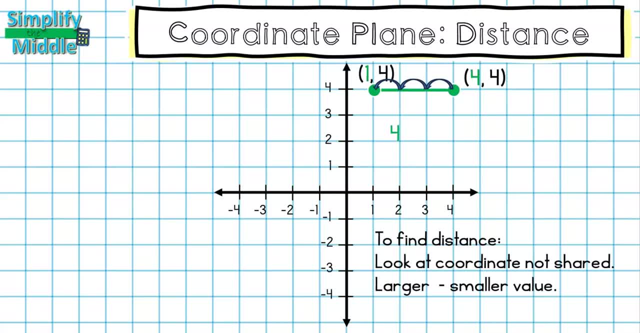 value. So here I have: 4 is bigger than 1, so 4 minus 1 is equal to 3.. And I know that that answer is correct because I do have a graph picture and I counted. but also I know this is correct because it is a positive number and my 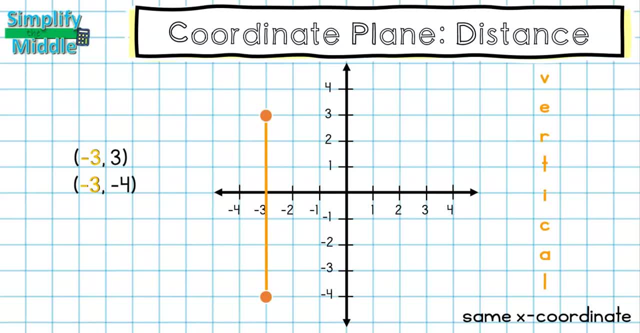 the same x-coordinate, they make a vertical line. Now that we understand the difference between them, let's practice trying to find the distance between them. So here I have two points: 1, 4, and 4, 4.. I automatically know that they are. 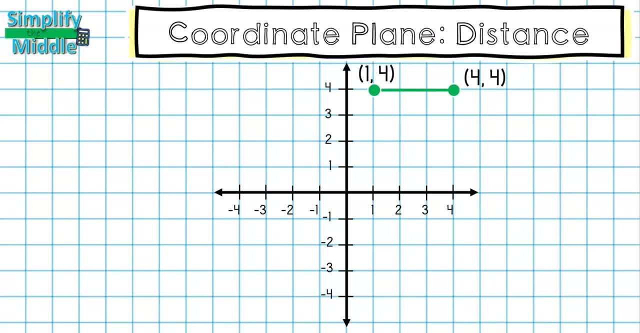 horizontal because I see them graphed. But what about if I don't see them graphed? So, because these ones are graphed, I do notice that it is going from left to right and I also can see from my ordered pairs. if I didn't have a picture of it, I 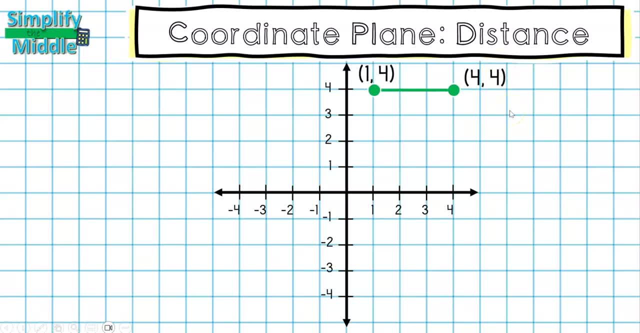 can see from my ordered pairs that the y-values, the y-coordinates, are the same. This means horizontal. Now to find the distance in a picture, I can just count that The distance between them. So this is 3.. So let's try another way to find the. 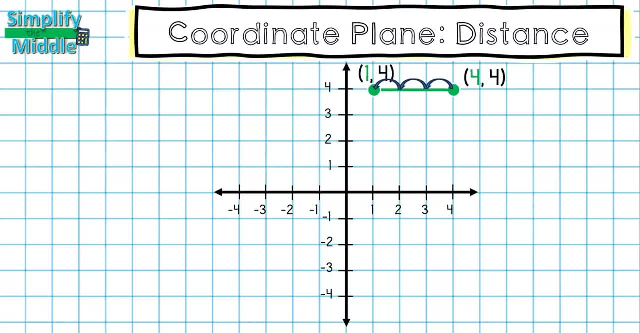 distance when I don't have the picture. So if I was to just have the ordered pairs To find distance, we're going to look at the coordinates that are not shared, In this case the x-coordinates. We will take the larger minus the smaller. 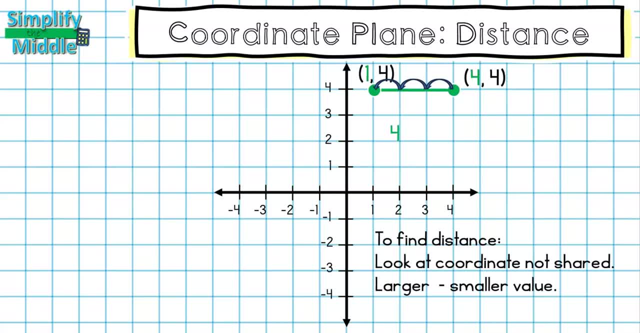 value. So here I have: 4 is bigger than 1, so 4 minus 1 is equal to 3.. And I know that that answer is correct because I do have a graph picture and I counted. but also I know this is correct because it is a positive number and my 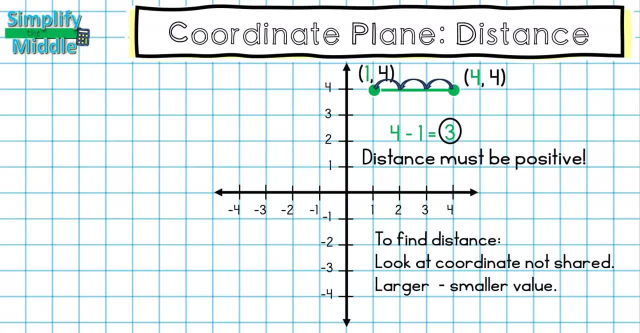 distance must always be positive. So if you get to the end of your question and you see that you got a negative number for an answer, then you know that you must have done something wrong, because distance must always be positive. Let's take a look at those points from earlier: Negative 3, 3 and negative 3, negative 4.. 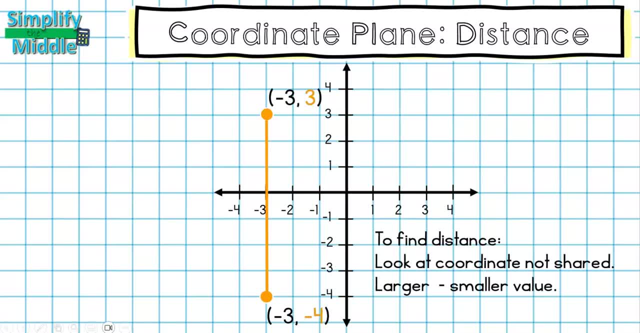 So here again, we can see that they have the same x-coordinate. And when you have the same x-coordinate, that is a vertical line, And I have my non-shared values as my 3 and my negative 4.. Because this is graphed, I'm 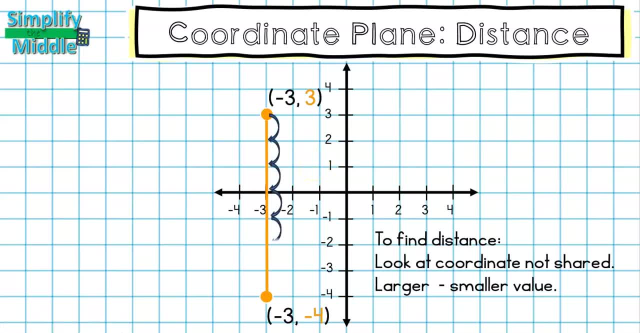 going to go ahead and count the distance between these. So as I count, I notice that I get 7.. And then I'm just going to go ahead and write out this problem the same way that I did the other one. Keep in mind that the higher up on the graph 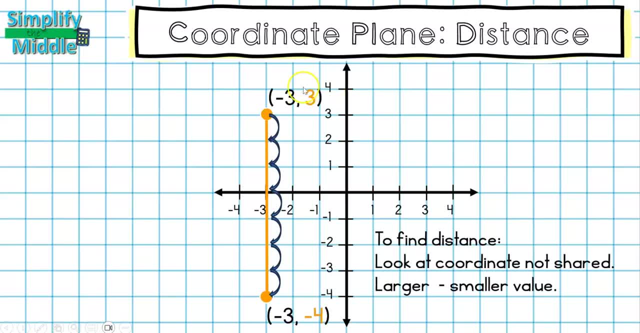 for a vertical line. the bigger the number, the more the number of the negative numbers. So I'm going to just write 3 and I'm going to keep the number there. Also, this is a positive and this is a negative. So that's how I can tell. 3 is bigger than 4 as well, So I'm going to 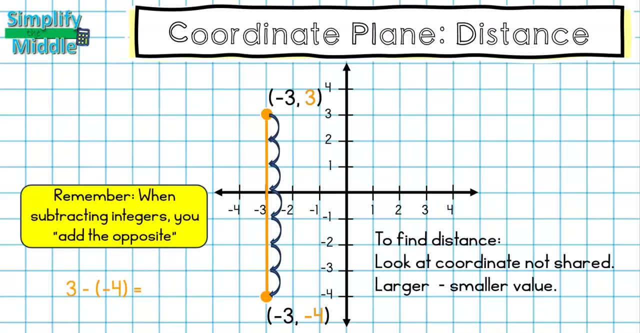 say 3 minus negative 4.. And I just put parentheses around it to keep it the problem a little bit more organized. And then remember, when you're subtracting integers, you're actually adding the opposite. So we don't subtract integers. 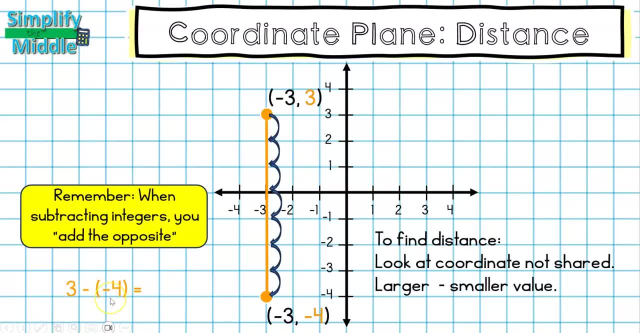 we just change it to add the opposite. So I'm going to keep the 3 the way it is, And then I'm going to keep the positive 4.. So it's actually 3 plus 4.. So my answer is 7. And I could confirm that from the picture of it being drawn and me counting. 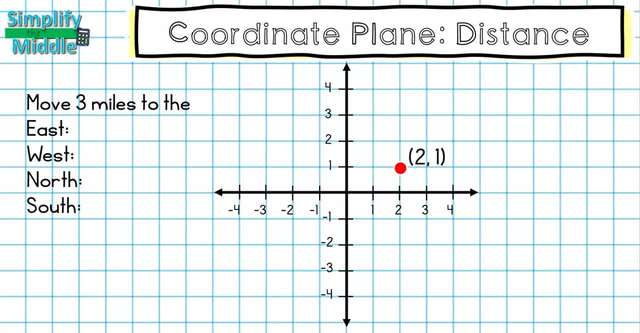 those, the distance of those units as well. So let's take a look at one last type of problem that you might see, And this is when you have cardinal directions. So let's say, here we are, at our point 2, 1.. And it tells us it wants us to move. 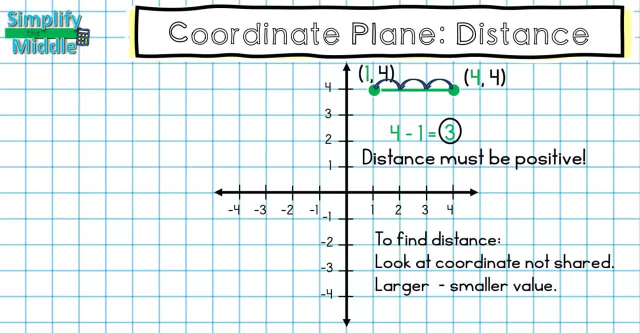 distance must always be positive. So if you get to the end of your question and you see that you got a negative number for an answer, then you know that you must have done something wrong, because distance must always be positive. Let's take a look at those points from earlier: Negative 3, 3 and negative 3, negative 4.. 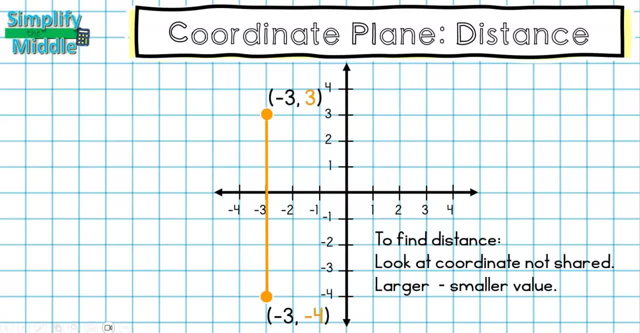 So here again, we can see that they have the same x-coordinate. and when you have the same x-coordinate, that is a vertical line, And I have my non-shared values as my 3 and my negative 4.. Because this is graphed, 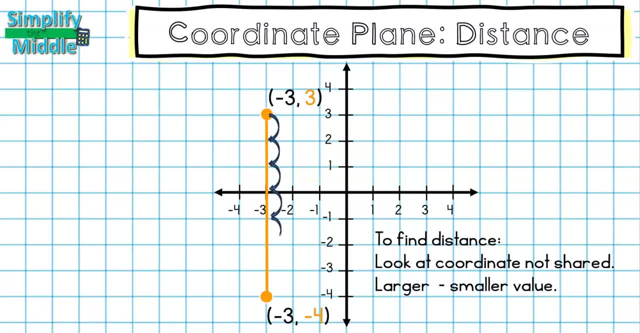 I'm going to go ahead and count the distance between these. So as I count, I notice that I get 7.. And then I'm just going to go ahead and write out this problem the same way that I did the other one. Keep in mind that the higher 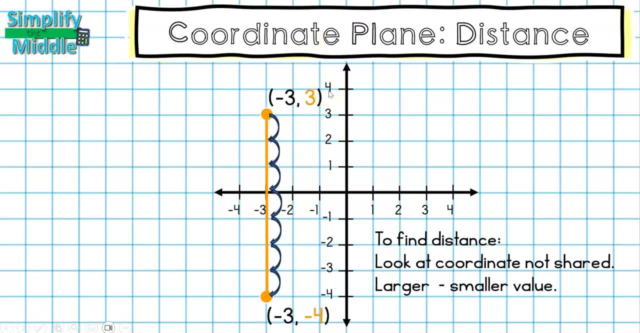 up on the graph for a vertical line. the bigger the number, the higher the number will be. So that's how I can tell that this is a positive and this is a negative. So that's how I can tell 3 is bigger than 4 as well. So I'm 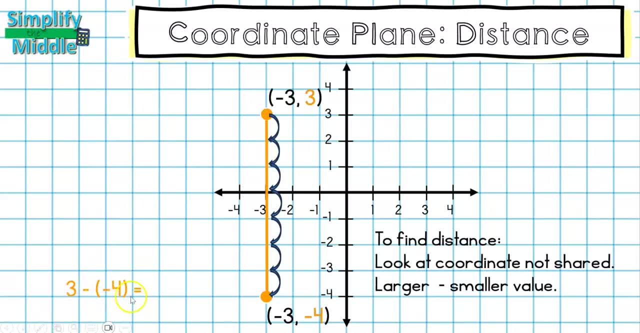 going to say 3 minus negative 4, and I just put parentheses around it to keep the problem a little bit more organized. And then remember, when you're subtracting integers, you're actually adding the opposite. So we don't subtract integers, we just change it to add the opposite. So I'm going to keep the 3, the 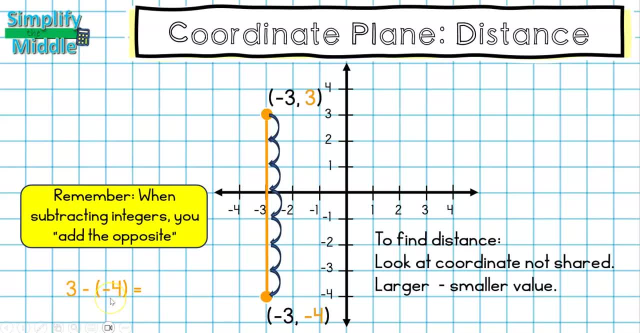 way it is. Change this to addition So it's 3 plus the opposite of negative. 4 is 4, so it's actually 3 plus 4. so my answer is 7 and I could confirm that from the picture of it being drawn and me counting those, the distance of those. 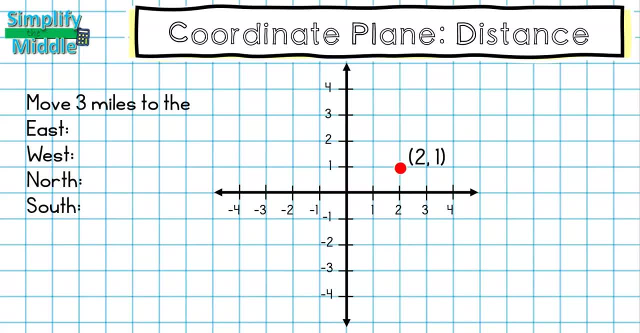 units as well. so let's take a look at one last type of problem that you might see, and this is when you have cardinal directions. so let's say, here we are, at our point 2, 1 and it tells us it wants us to move 3 miles, and we're assuming- 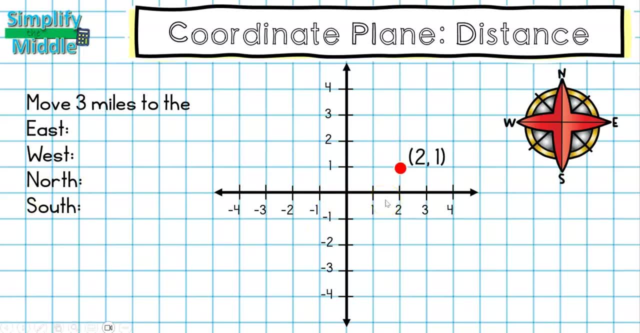 that each unit here is a mile. it wants us to move 3 miles to the east, west, north and south, so I'm gonna have four different ordered pairs. that represents each of those movements. the first thing that I'm gonna do, I went ahead and put together a little table that makes this really easy for me to know what I'm. 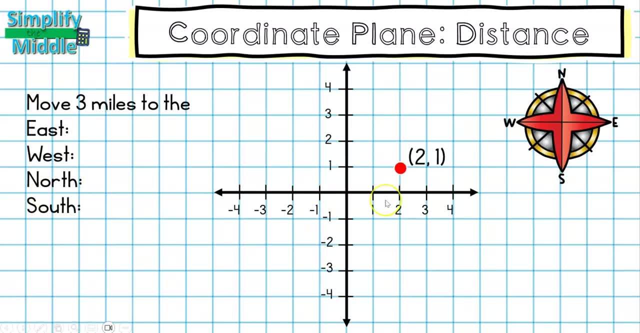 3 miles And we're assuming that each unit here is a mile. It wants us to move 3 miles to the east, west, north and south, So I'm going to have 4 different ordered pairs. that represents each of those movements. The. 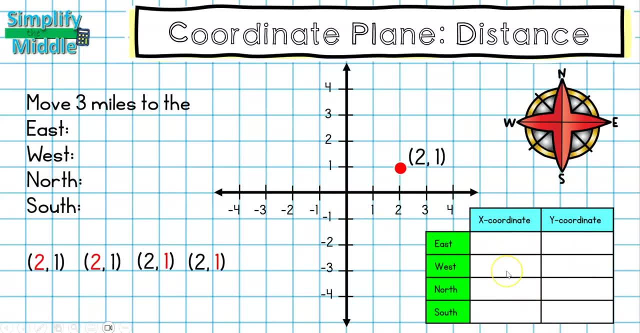 first thing that I'm going to do, I went ahead and put together a little table. that makes this really easy for me to know what I'm doing for each of the coordinates. And the second thing that I did is I just went ahead and wrote out. 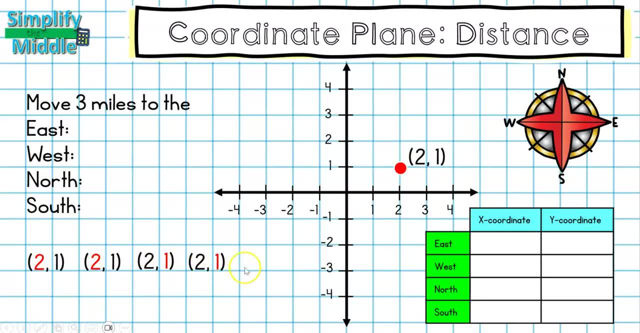 my original point 2, comma 1.. And I'm going to do my math down here. So if I go to the east, east is this direction. As I'm going this direction with my point, I notice that my numbers for my x value, my x coordinate, is getting bigger, But nothing is happening. 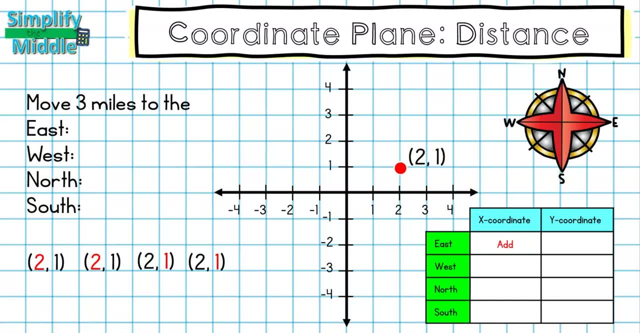 to the 1.. So to go east, I'm going to add that 3. And I'm going to keep my y coordinate the same. So my new point: if I was moving from 2, 1 to the east, 3 miles. 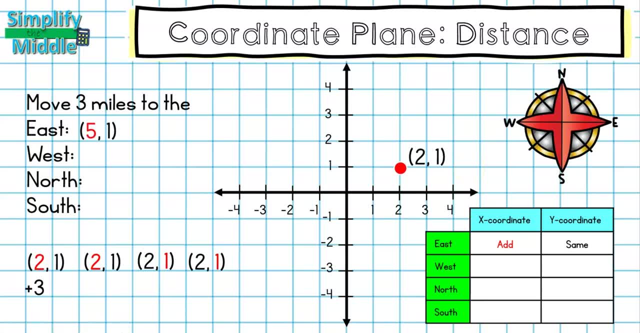 would be 5 comma 1.. To move to the west: west goes this direction, So I can see I'm moving over here and I'm moving 3.. So I'm actually going to be subtracting, but I'm only moving on my x coordinate. So I'm going to subtract 3 from 2. And I'll keep. 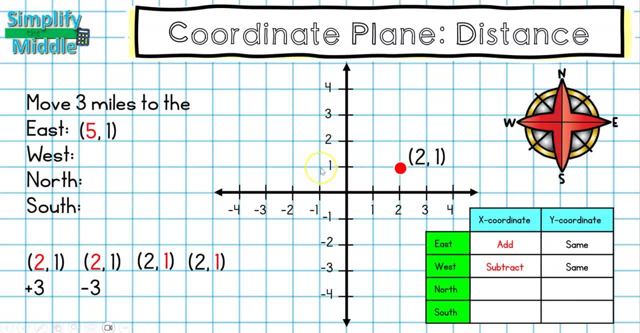 my y coordinate the same, because it didn't go up or down, it just went to the west, And 2 minus 3 is going to give me negative 1, 1.. Next, to go north, I'm going up, so I'm going to go up 3. So I'm adding, making 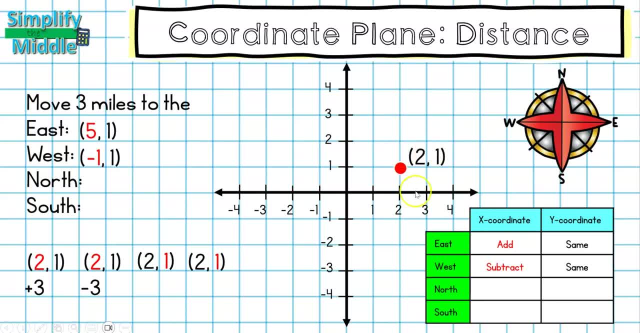 that 2 bigger. I'm sorry, I'm making the 1 bigger In this case. I'm not going to do anything to the 2, so notice how it doesn't have a color, And the reason why is because my x is going to stay the same. I'm going to stay on this line. 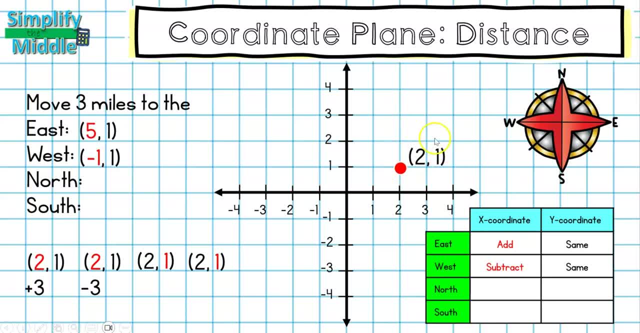 I'm just going to go up on that line and I go up 3.. So it's my y that I'm going to add to. So I end up with 2 comma 4.. Then, finally, if I want to go south, I'm going to be going down, but I'm still staying on the same x-coordinate, so that 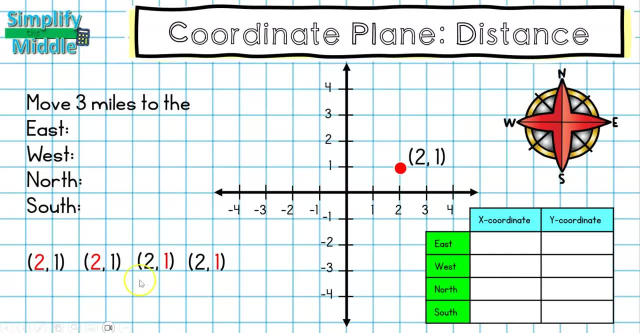 doing for each of the coordinates. and the second thing that I did is I just went ahead and wrote out my original point 2, comma 1, my original ordered pair, and I'm going to do my math down here. so if I go to the east, east is this direction, as I'm going this direction with my 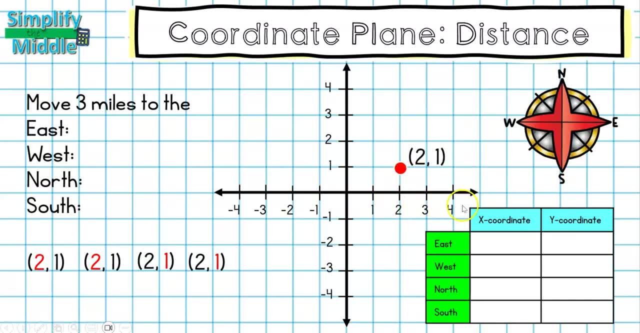 point, I noticed that my numbers for my X value, my X coordinate, is getting bigger but nothing is happening to the 1. so to go east, I'm going to add that 3 and I'm gonna keep my y-coordinate the same. so my new point: if I was moving from 2 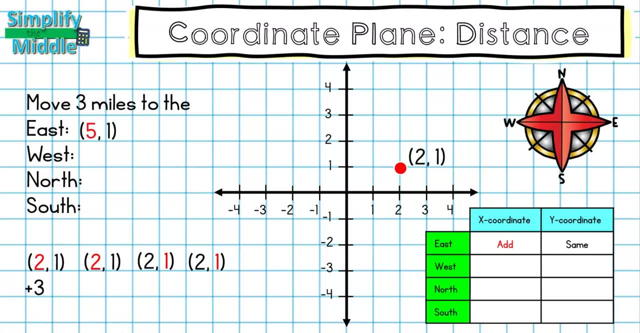 1 to the east. 3 miles would be 5 comma 1. to move to the west. west goes this direction. so I can see I'm moving over here and I'm moving 3, so I'm actually going to be subtracting. but I'm only moving on my X coordinate, so I'm going. 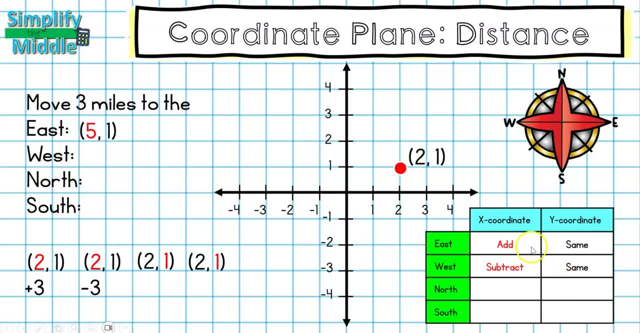 to subtract 3 from 2, and I'll keep my y-coordinate the same, because it didn't go up or down, it just went to the west, and 2 minus 3 is going to give me my negative 1, 1. next to go north, I'm going up, so I'm going to go up 3, so I'm adding. 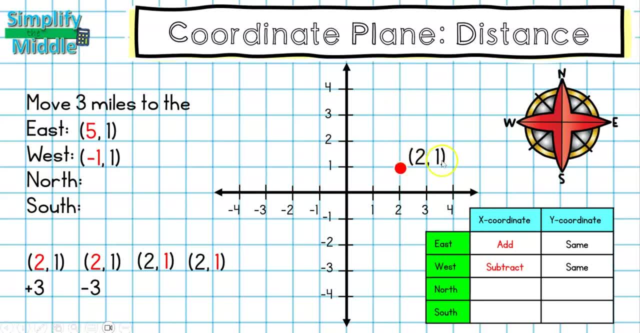 making that 2 bigger. I'm sorry, I'm making the 1 bigger in this case. I'm not going to do anything to the 2, so notice how it doesn't have a color, and the reason why is because my X is going to stay the same. I'm going to stay on this. 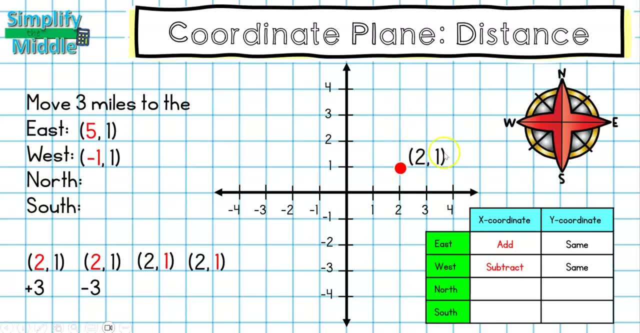 line. I'm just gonna go up on that line. I'm gonna go up 3, so it's my Y that I'm going to add 2, so I end up with 2 comma 4, and then, finally, if I want to go south, I'm going to be going down, but I'm still. 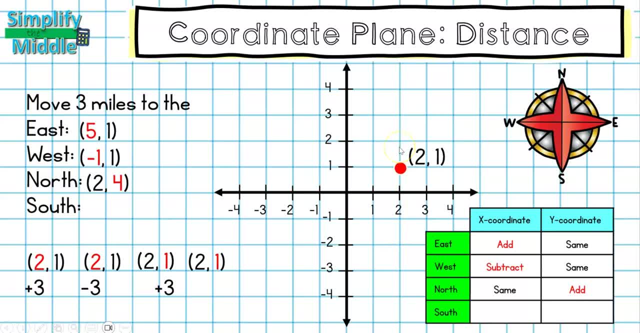 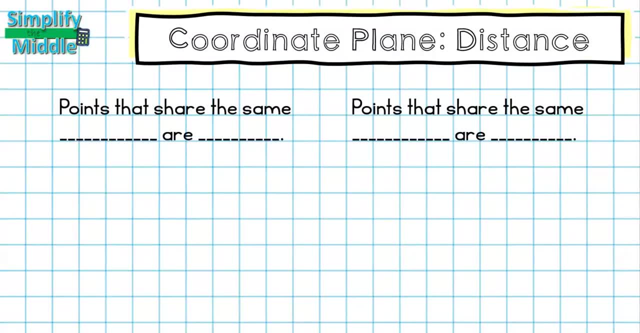 staying on the same X coordinate. so that stays the same and I will be subtracting the 3, so I end up with 2 comma negative 2. let's recap: points that share the same y-coordinate are horizontal and points that share the same X coordinate are vertical. finally, we know to find the distance of points.